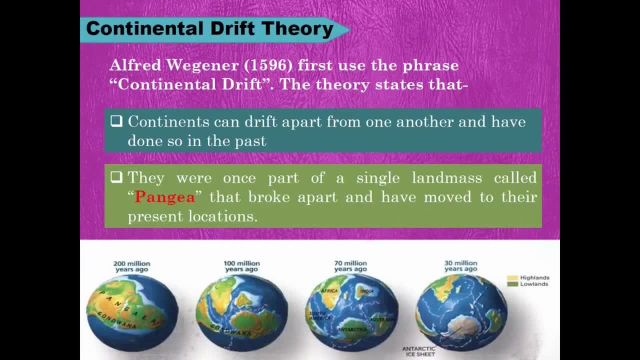 So first of all, we are going to talk about the continental drift. So what is continental drift? So this phrase continental drift was first used by Alfred Wegener. He was a famous geoscientist and he denoted the continental drift such as that there was once, probably 200 million years ago, all the continents that we see today were not exactly in the same place as they are in their current state. 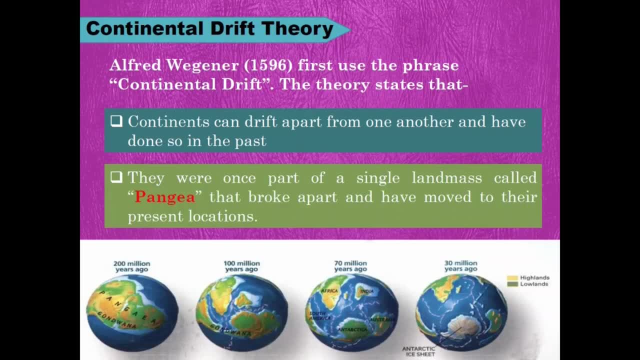 So it is supposed that all of them were in one single continent, which is a supercontinent known as the Pangaea. But over the span of time they have changed. They have tried to shift from one another and tried to break up and move away from each other. 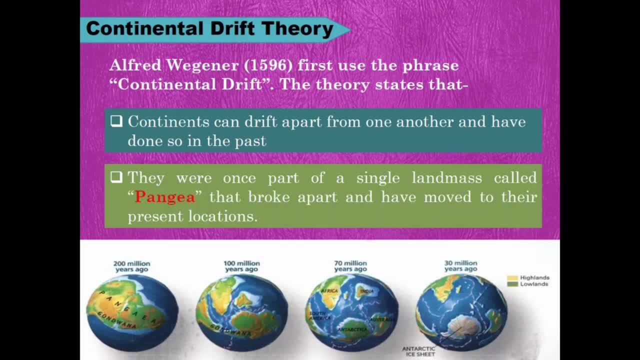 And over the last 200 million years, and from that time till now, they have reached their current state And this is still going. And this happens because of some internal processes that are ongoing beneath or inside our Earth's crust, or inside our Earth's internal. 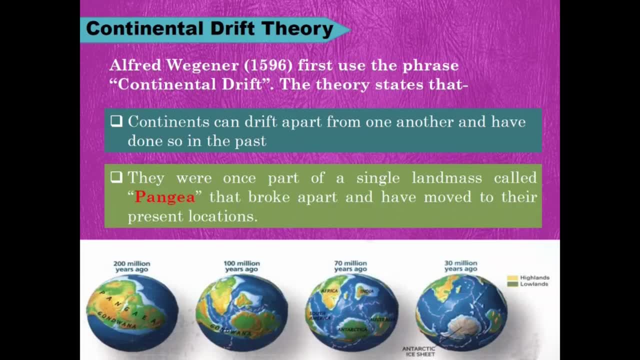 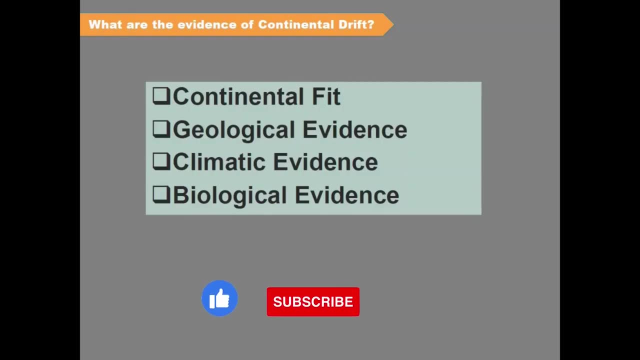 So we are going to talk about that later in this lecture. So now moving on, what are the evidence that supports the continental drift theory? So there are a lot of evidence, but in this lecture we are going to talk about the main four evidences. 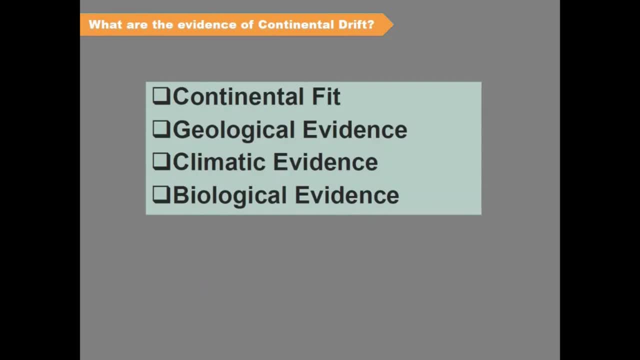 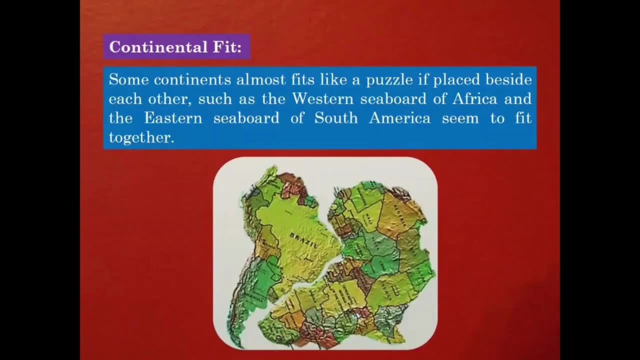 The first one includes the continental fit theory and the geologic evidences that are available, the climatic evidences and finally the biological evidences. So if we go to the continental fit, So if we see that some continents almost feels like a puzzle if they are placed beside each other in an organized way, 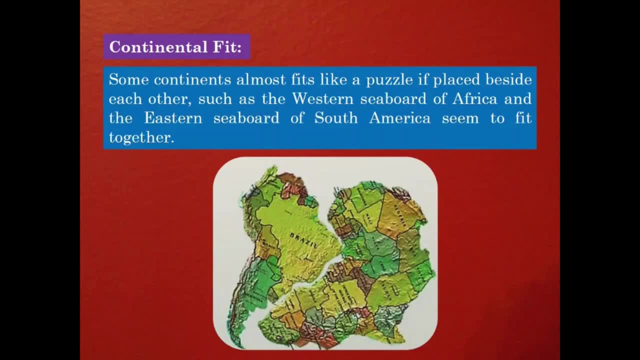 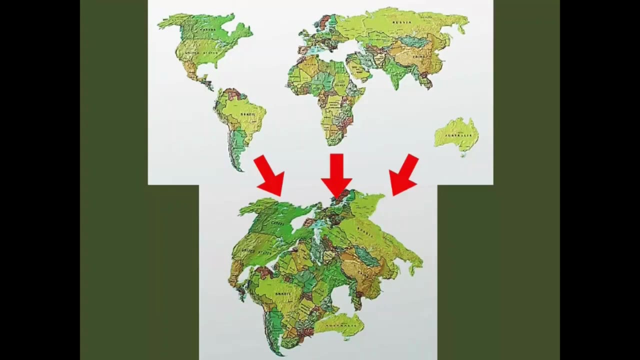 For example, if we take the western seaboard of Africa and the eastern seaboard of South America, we can see that both of them looks their borderline looks exactly like they were just broken from one another like a puzzle. So if we move on, so now here in this picture we take all the continents in their current state. 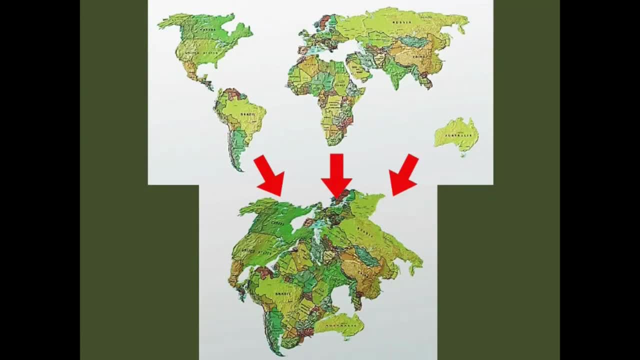 And if we try to fit them in an organized way, we'll have something like this in the bottom of my slide. So this very well supports the idea of the pangaea. Now the second theory and second evidence is the geological evidences. 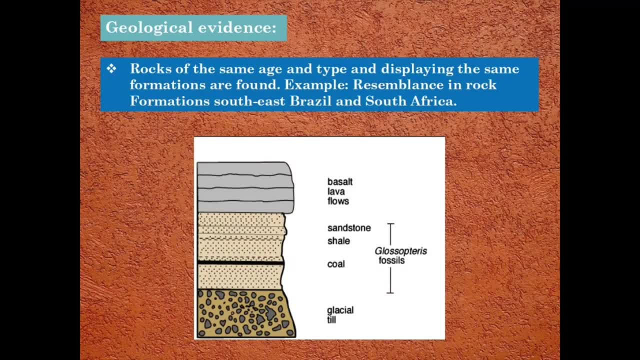 For example, rocks of the same age and time and displaying the same formations are found in different parts of different continents, for example, rock formations in the southeast Brazil and south West Africa, for example. not Brazil and Africa, but horizon, imagine. So these are the threerd evidences for geological evidences. 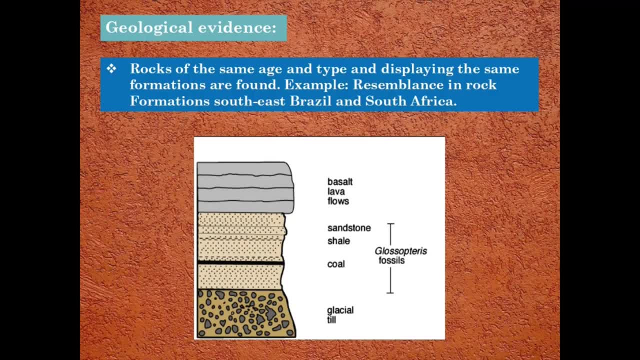 For example, rock formations in the southeast Brazil and Southeast Africa, for example. now Brazil and Africa, for example, are two different continents, but exactly same kind of formations have been found in both the continents. so this is something like if the climatic conditions, if the depositional and erosional sequences are not exactly the 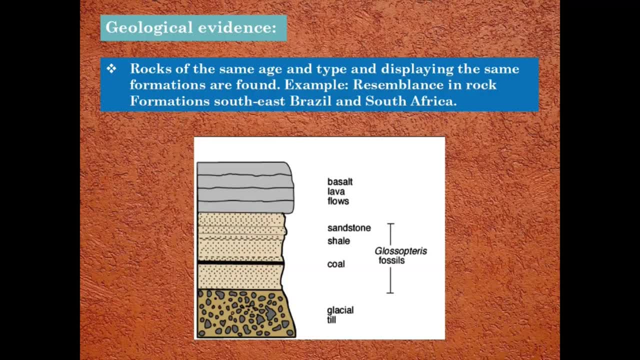 same. this is never possible in basic geological terms, but since we have found it so it means that maybe these two continents were exactly one continent at one period and they were run by the same kind of physical environments and, as a result, their formations were same. so similar thing goes for other birds also. 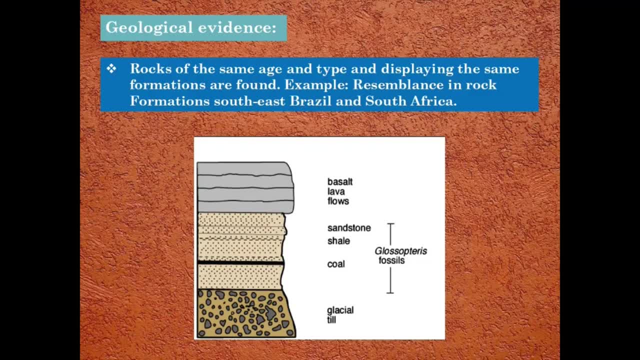 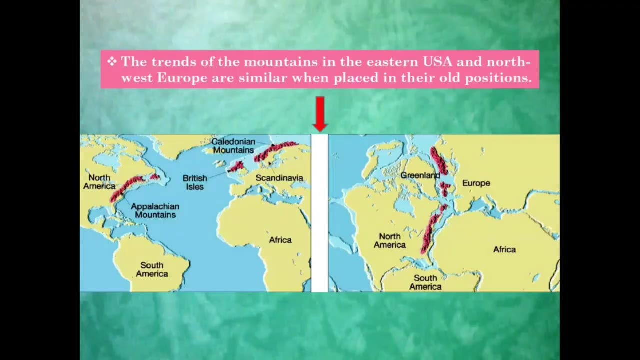 many other same formations have been found in other continents that show this kind of similar formations. that is also an evidence, which is known as the geological evidence of continental drift. Now, if we look at this picture you'll see, Down below is an example of an Eurasian winged nailed cliff of debut and expression of theòn digital inherently changes of continental drift. as aiza boleh birosab Garcia, that is also evident, which is known as the geological evidence of continental drift. now, if you look at this picture we will see. 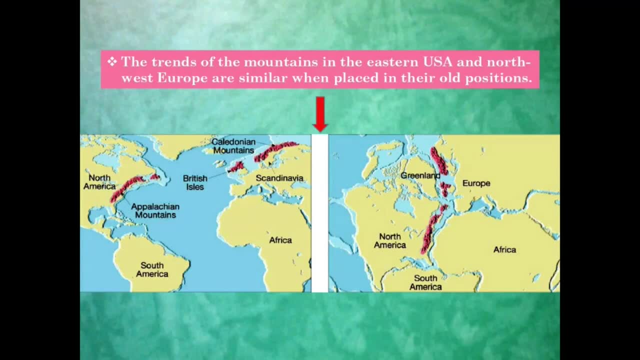 Aka into the lower. worse nowsl the ground is alive. voyages- so we discussed over graphed 1990- also suggest that in North America the famous Appalachian mountains, and if you go to the Scandinavian you will find the Claredonian mountains and the British. 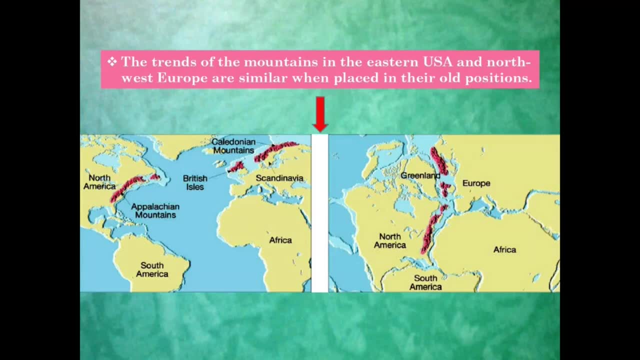 Isles mountains. so if, when we fit all the trees, that we are gonna get something like this, something, this long stretch of mountains, the best part is they all have the same kind of depositional structures. so this supports our idea that the continents are also fitting and this entire stretch is. 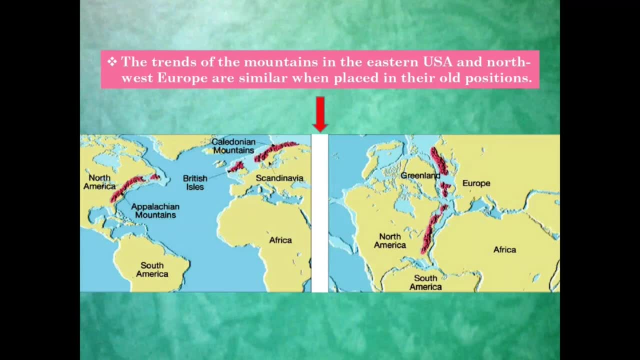 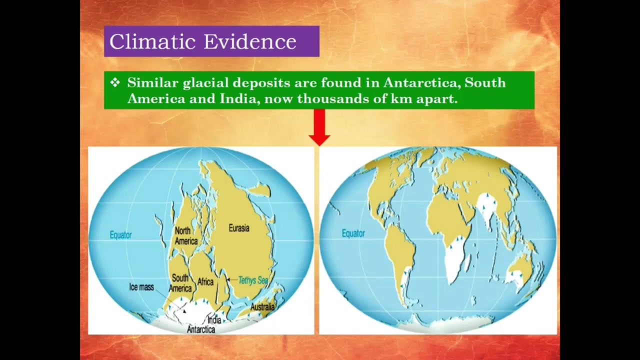 containing the same kind of formations. So maybe, maybe, billion or billion years ago in the past, all these continents wire together. Now moving on our third evidence, that is, climatic evidence. So similar glacial deposits are found in Antarctica, South America and India, now thousands of. 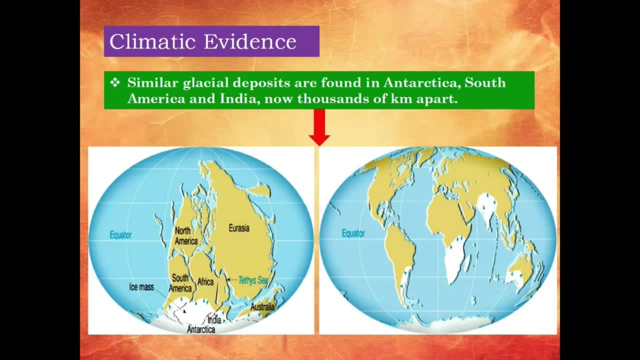 kilometer apart these continents that I just mentioned. they are like thousands of thousands of kilometer apart. so glacial deposit found in india sounds a little bit weird that india is not somewhere where you can actually find glacier or glacial deposit. also in south america there is not the same antarctica. yeah, we can say that in antarctica. 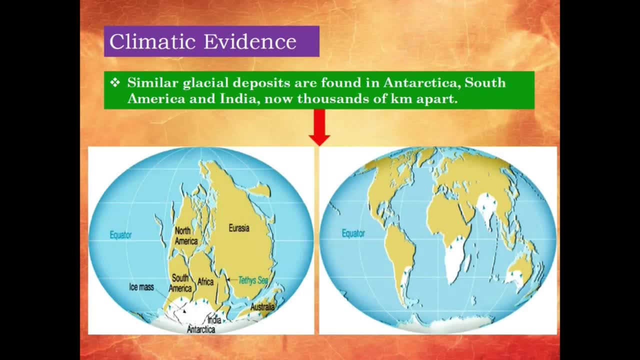 we can found the glacial deposit. but what about the other two continents? so this is another theory that suppose, maybe, maybe at one time- you can see in my picture in the left of the slide- that maybe in one type- india, antarctica and south america, they were all together and during that climatic 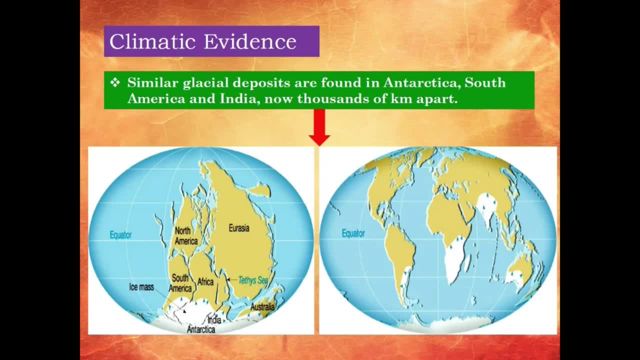 conditions. they all had the glacial deposits and maybe in the after the post, inter, post glacial integration period they moved away from each other still, but still the formations are there. the glacier deposits are there. that supports our theory of climatic evidence. and the fourth evidence is like the biological evidence. so how? 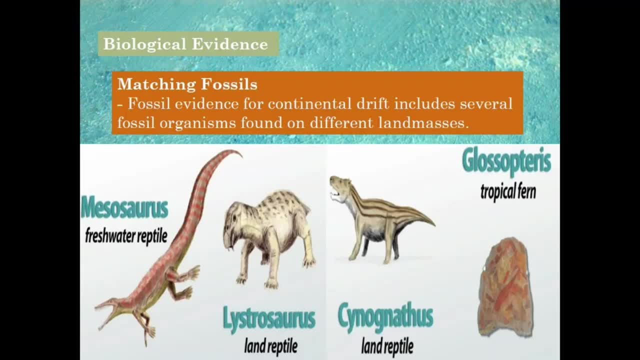 do you determine the biological evidence is by matching the fossils. you see, different continents have contained same kind of biological evidence and now you know that, if we consider animals, especially animals can only breed with same species if they're together in one continent. okay, so, for example, listosaurus sinonotus- these two are land-based animals. on the other has mesosaurus. 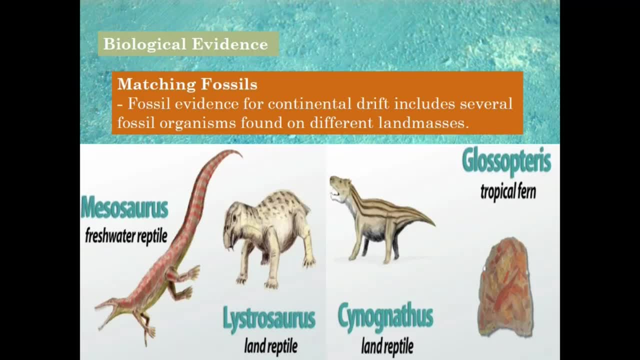 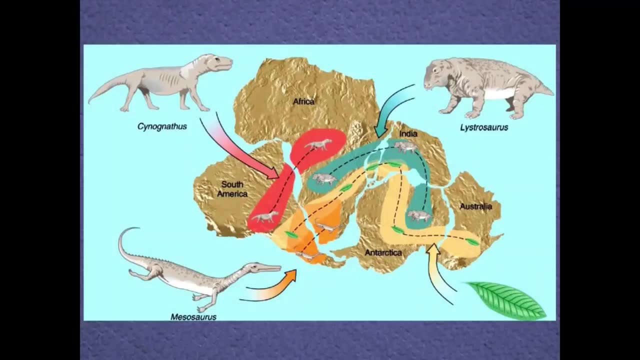 is a freshwater reptile and glossopithecus is a tropical farm, which is a like a floral species. now, if you see this picture, sinophagus and listosaurus. they were both found in india and antarctica and in africa, for example. these are species. 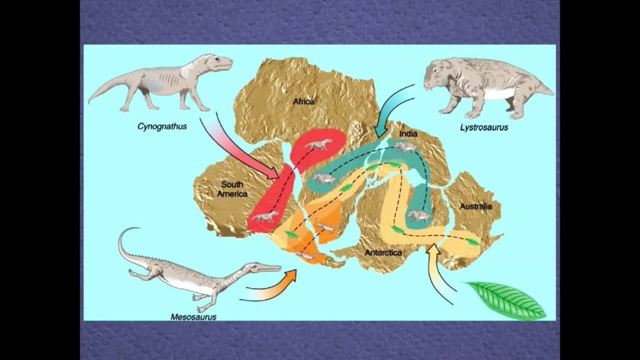 that do not know how to swim. so if the continents are not together, how in the world it is possible that they cross the sea without knowing swimming? so if you have to do a migration from one continent to another continent, then you definitely need to swim. so this was not possible in case of 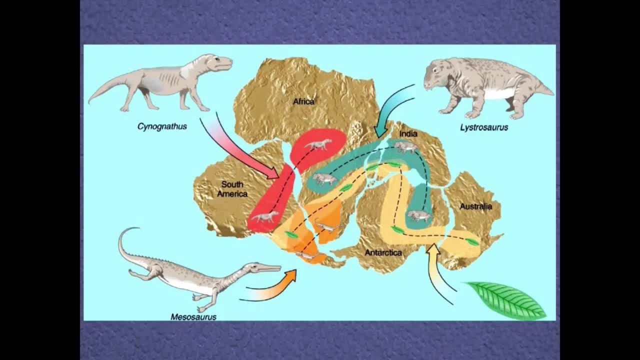 listosaurus and sinogathosaurus. so this idea is only possible if all the continents are together, so only that time they can make the migration from one part to another, and maybe during making their migration they were there and that after hundreds of hundreds of billions of millions of years the continent shifted away, but their fossil remains are still in the same place, exactly the same way. same goes for the mesosaurus. mesosaurus are like freshwater reptiles: they can swim, but they cannot swim in saline waters. and how in the world? 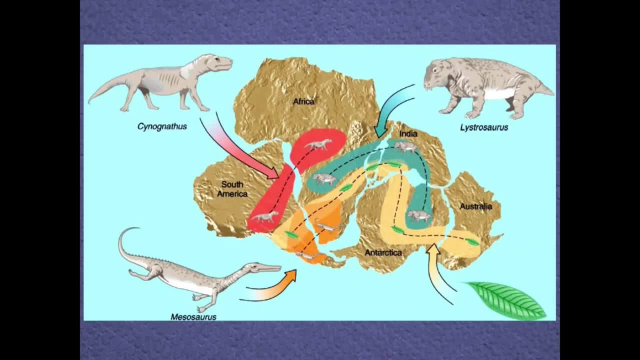 mesosaurus fossils are found all above south america and africa. that is impossible. they cannot survive in saline water, so definitely these continents have to be in the same place and one in the time period of the formation of the entire art and between their current state. same goes for 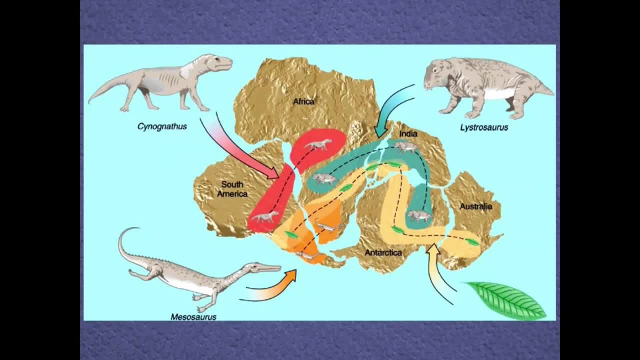 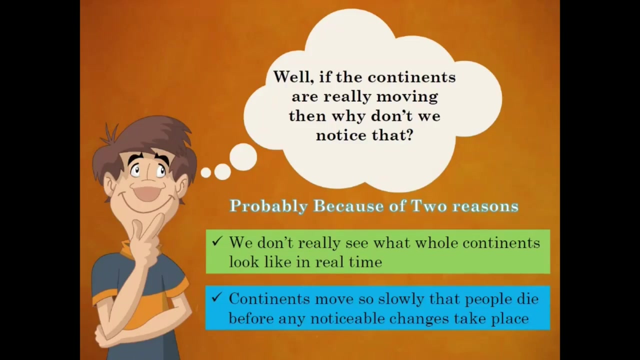 the glossopteris, if you see, this floral species have been found in all of the continents. so exactly the same point that if, unless they were, the continents are together, this migration and this spread of this species was quite impossible. okay, now there is a question. okay now, some of you might think: well, if the continents are really moving, then 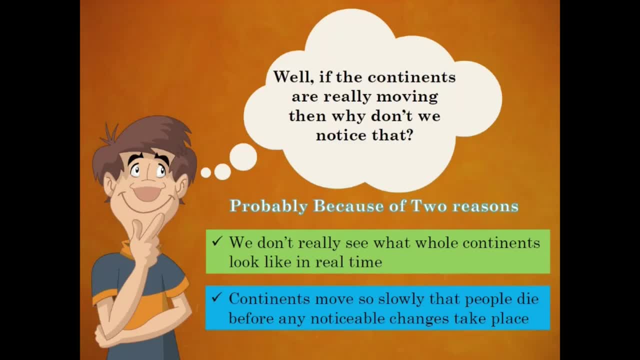 why don't we notice that? probably because of two possible reasons. we don't really see what whole continents look like in real time. comparing to the continents, we are really small human beings, and also the continents move so slowly that by the time you age, by the time you die, there is like only centimeters or like meters. 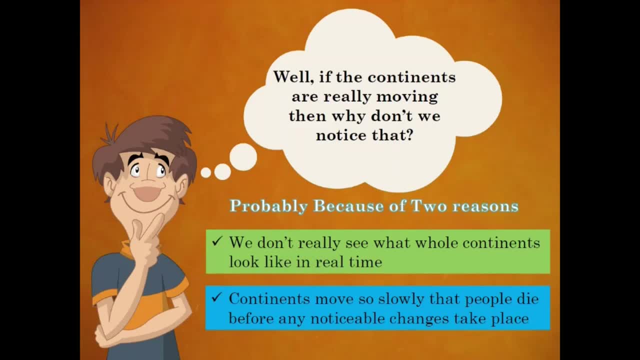 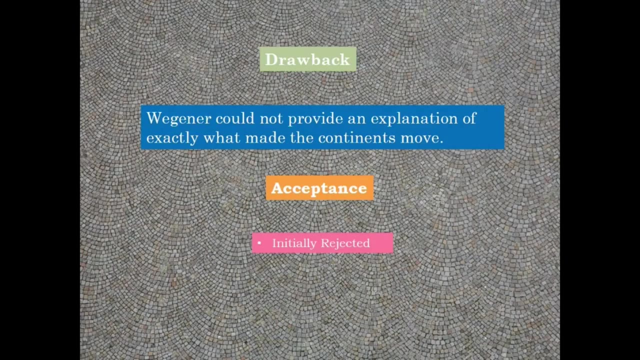 which is like, not possible for a human being to see her, he's or her whole life in front of one continent and measure the movement. so by the time we can actually measure anything, we don't stay alive. so that is another theory. now, uh, this theory, like every, 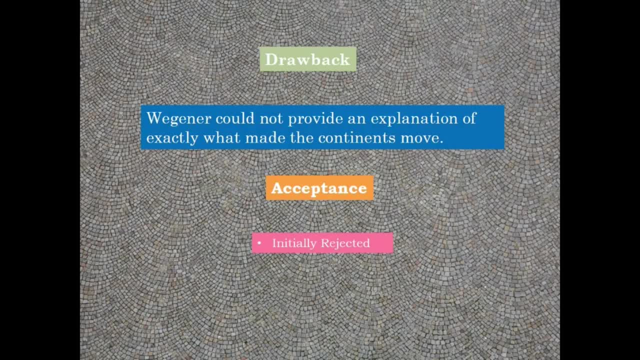 other theory. this theory has some drawbacks. so, although wager could not either describe this continued theory- but región could not provide an explanation of exactly what making a table's- but we're doing the best in it- is that wagner could not provide an explanation of exactly what made talented swiss. conttilical- 這個必以菠溝的場 thaver at well, which is that they nearly survived heather. if one of these things iranians are learned at their home and afraid of, is more likely they will survive wings or after reducing the pepper when they are eating蜜蜂. 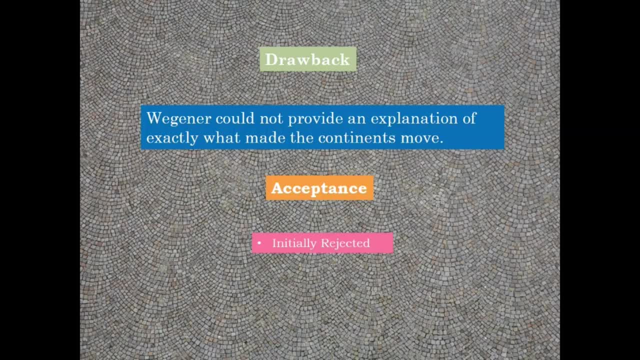 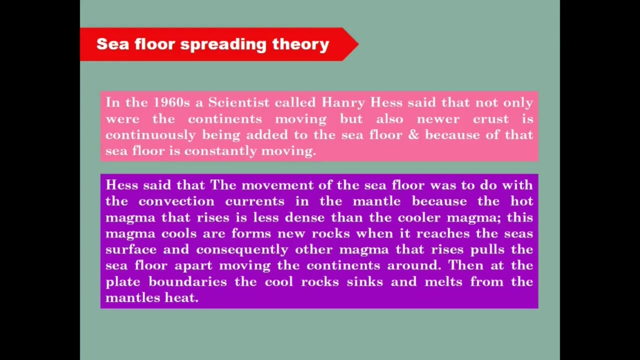 what made the continents move. so that is why there is a big question about the acceptance of this theory, and this theory was initially initially back then when he claimed. this was rejected. but later there was another theory came the sea floor spreading theory. in 1916, scientist called henry hayes said that not only were the continents moving, 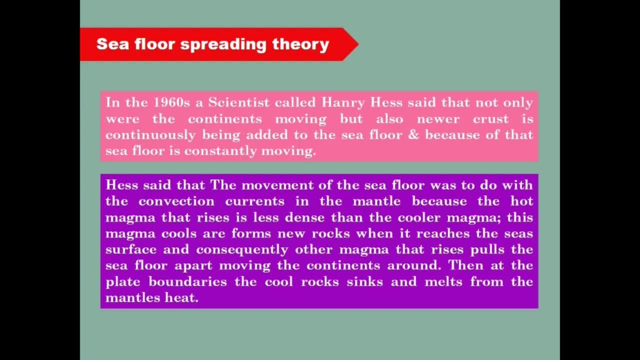 but also newer crust is continuously being added to the sea floor and because of that sea floor is constantly moving. he has said that the movement of the sea floor was true with the convection currents in the mantle, because of the hot magma that rises is less denser than the cooler magma. 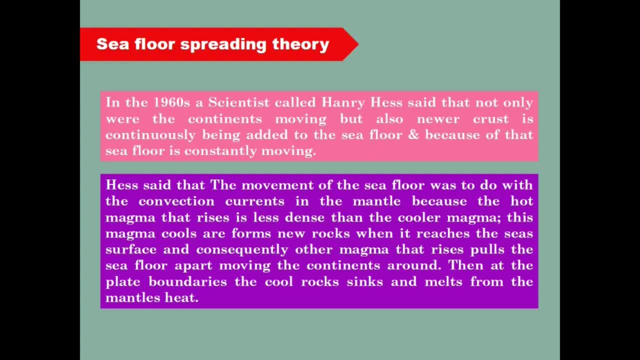 and these magma cores are forms, new rocks when it reaches the seas and surface, and continuously, other magma that rises, pulls the sea floor apart, moving the continents around. so, for example, this movement, we know the convection. so because of the convection of the mantle, there are two layers of 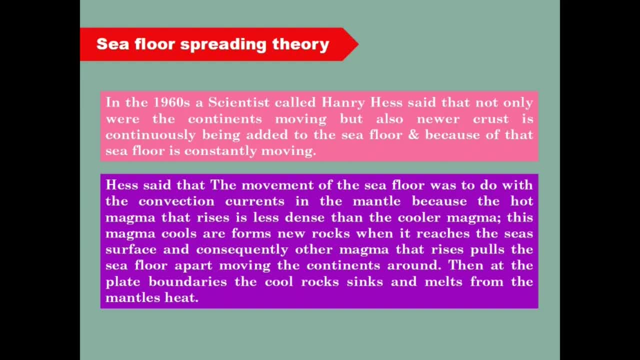 i will not say two. there are multiple layers of magma in different kind of variation of temperature in our mantle and, as the rule of physics, when you have different kind of temperature, the cooler temperature liquid will flow upwards and the water temperature liquid will flow downwards, creating a convection, creating 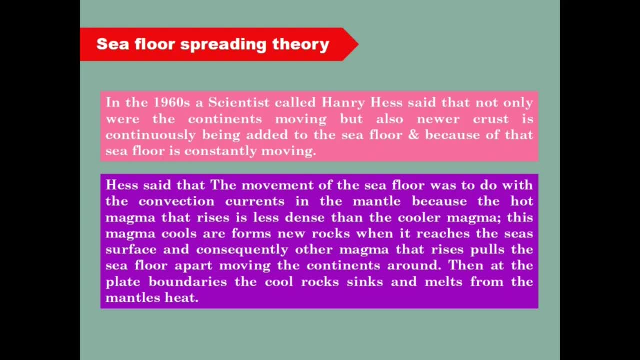 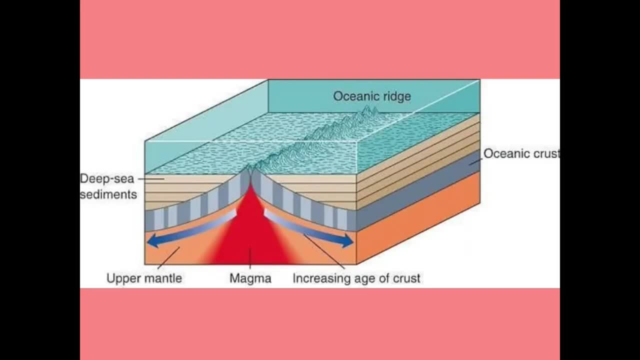 a circular convection and because of the circular convection, the grants do the movements. and now, if you see this picture, this will explain how this works. so when the currents, when both the circular movements are apart from each other, they will tear the continents apart from each other. so that's how the continents can. 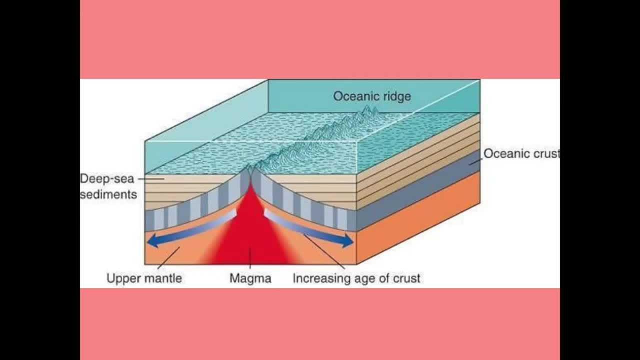 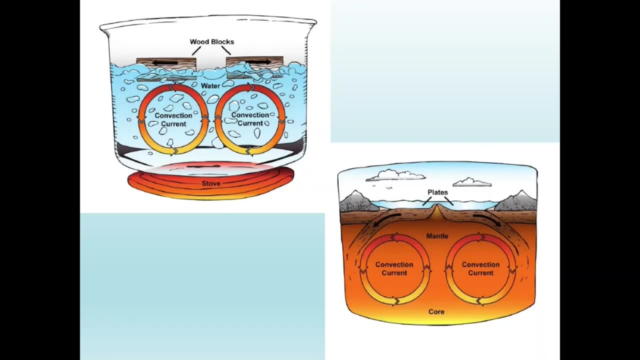 actually move and sea flow is spreading supports this idea. now you can test this theory at your home also. if you take a bowl and if you keep two pieces of food in the water of the bowl and you start boiling the water, the more the temperature increases, there will be a convection current. 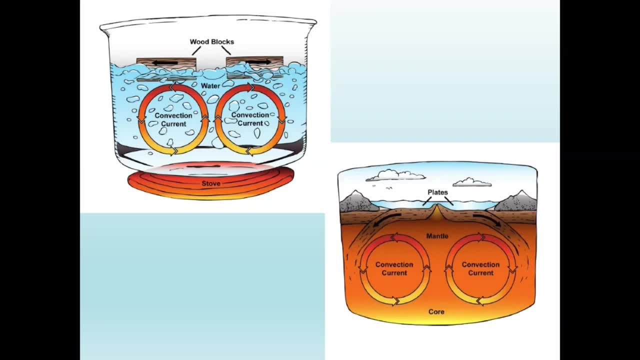 created within the bowl or within the thing that you are using, and you will see that both the roots will draw away from each other in within the liquid of that bowl. so exactly the same case happens in our mantle. so these two scenarios are majorly comparable. now not only they move away from each other, 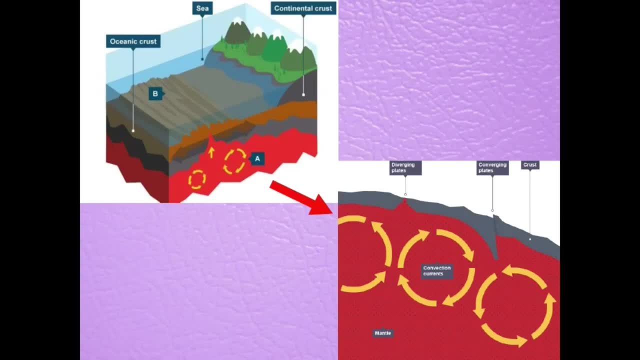 but the convection, the way of the circulation of the both two currents can be towards each other's also, and when that happens, continents will move towards each other rather than going away apart from each other. okay, so both the scenarios are possible and both the scenarios are happening, and both of these scenarios supports. 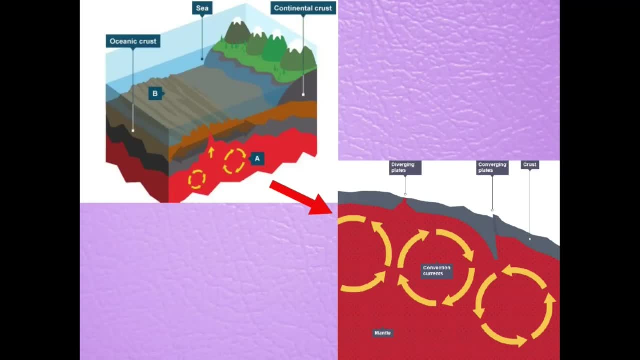 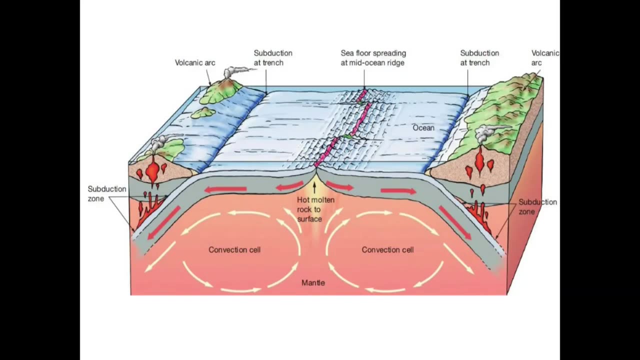 the previously rejected continental drift. so here is a picture that clearly depicts that how the continents are moving and you can see in the middle the convection is towards each other. that is tearing the continents apart to are steering the ocean increased apart. as a result, hot molten magma is. 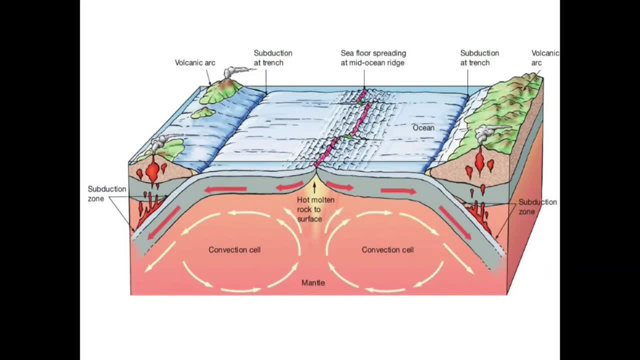 coming upwards and with touch of water and in contact water they are cooling down immediately, forming newer crust. on the other hand, if you go both the sides, you can see the previously generated crust are going down towards each other, because when two continents are moving towards each other, the denser 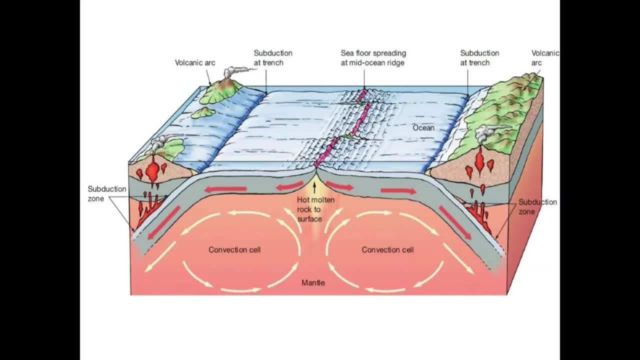 plate, that is normally the oceanic plate, which is denser- goes beneath the landing or the terrestrial plate and, as a result, it subducts, and it subducts into the hotter, hotter place of the mantle and it again turns from solid to liquid and forms new. 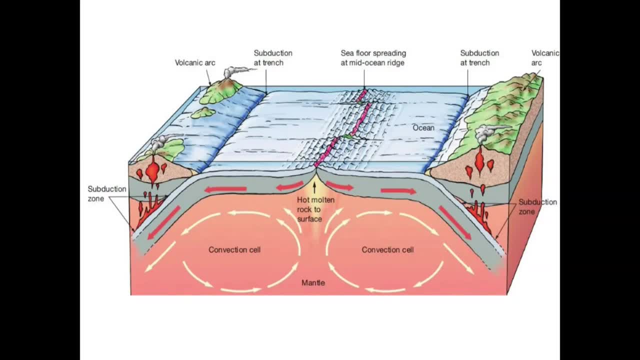 magma and because of the subduction, not only that, the oceanic crust gets molten. on the other hand, the earth plate or the terrestrial continent that is on the land, part of our world that gets uplifted. so there are both the cases happening and this is a strong support of the previously rejected continental 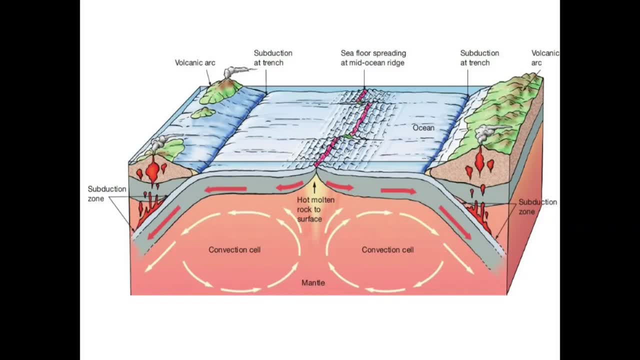 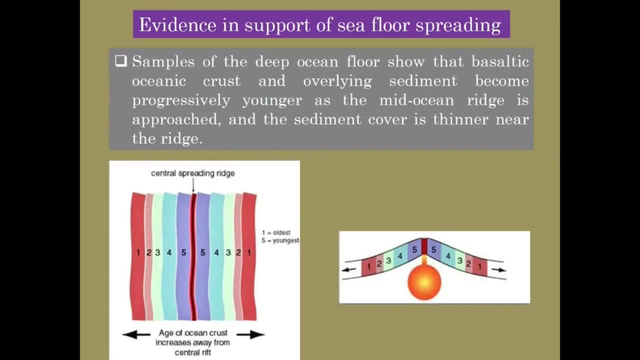 uh theory. so you can see say that the continental drift was supported by the sea. flow is spreading. so then, after more research there is, there are many more other evidences that came out, and another one is the age of the oceanic crust. you can see if we measure from the plates or the position. 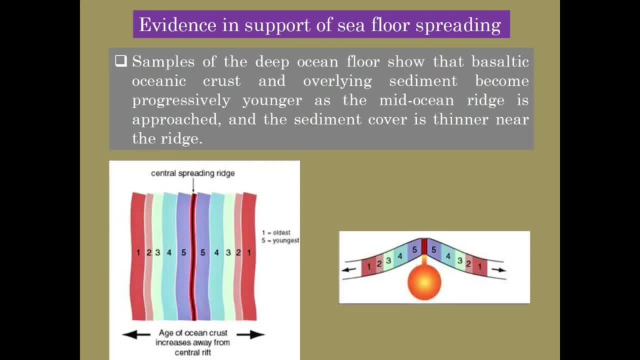 from where we think that the plate are spreading towards each other. so if you take the middle point as a line, as a standard of zero, and you go in the left and you go in the right, you will see that there are specific plates or specific portions of that plate, exactly the same amount from the moving. 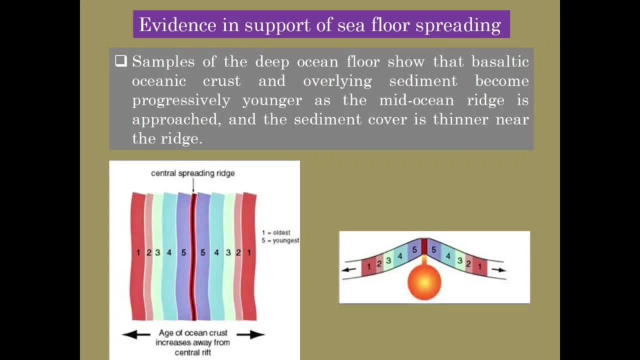 places who have the similar age, in the right and in the left. for example, if the position red line, red and black line in the picture is our position of moving of the plates from each other, then we go left one kilometer and we go right one kilometer from the position. we will find similar kind of plates and we 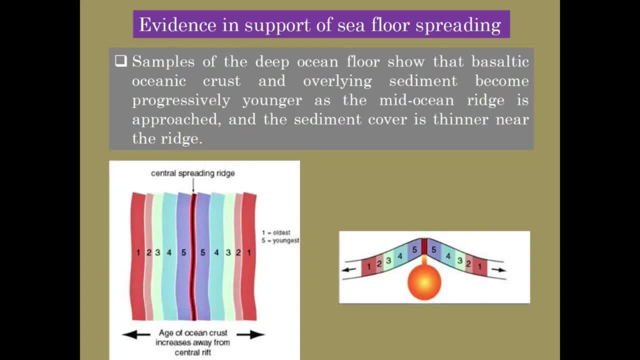 go right, one kilometer from the position, we will find similar kind of crust, similar kind of oceanic plate that has the composition and age of exactly the same kind of rock formation, and same thing happens in both the sides. so, and the closer the portion, the younger it is, and the distant the 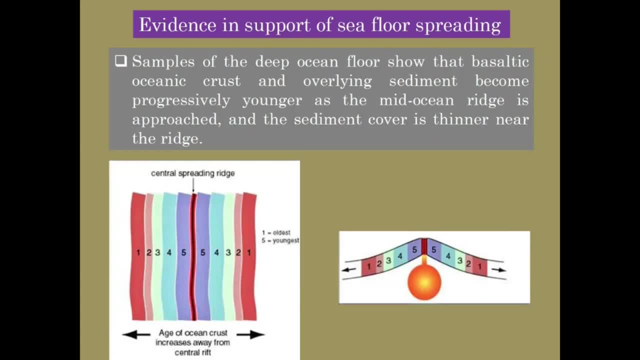 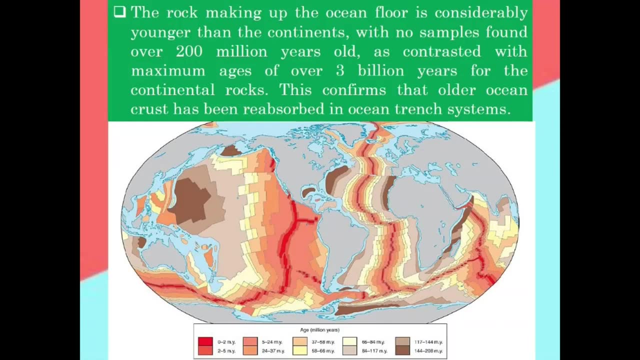 portion from the place of movement, the older the rock formation is. so if you go to the, if you take it 2d version of the whole world and if you take all the spreading zones or all the places where plates move away from each other, we will. 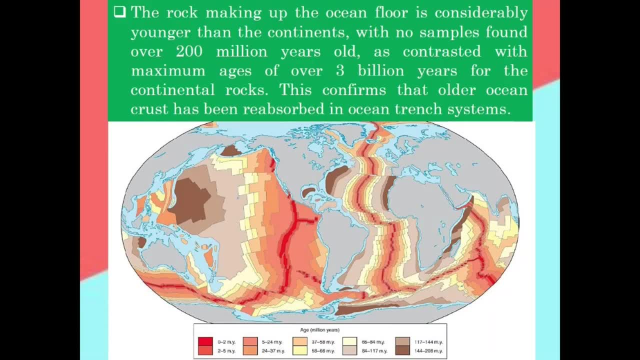 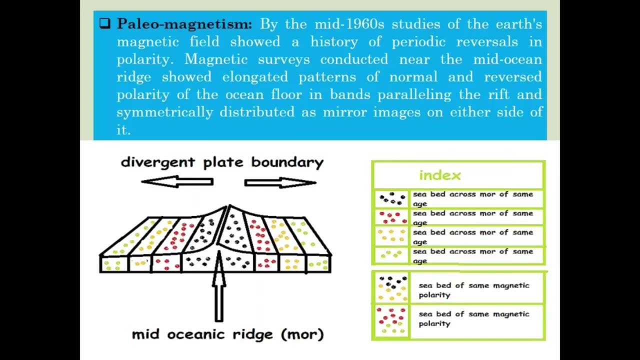 find something like this that will support the idea of similar aged rocks. now, not only that their age and composition will be similar, but there is another interesting fact, as we know that when one specific formation of rocks generates in one place, they have a polarity, they have internal polarity. 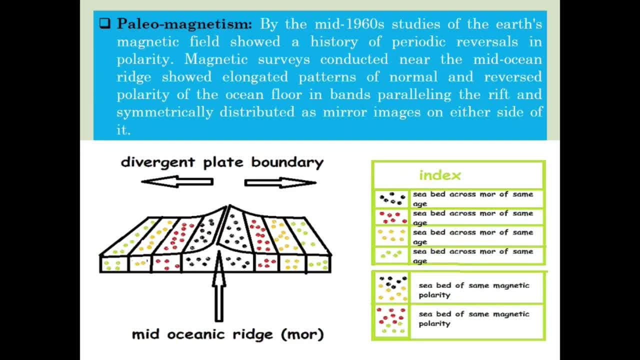 so not only their age- and they are distant from the source- is same, but you will see that each will contain the same kind of polarity. for example, the younger rock, if there is positive and negative polarity from north and south, the later one, the older one which is adjacent to 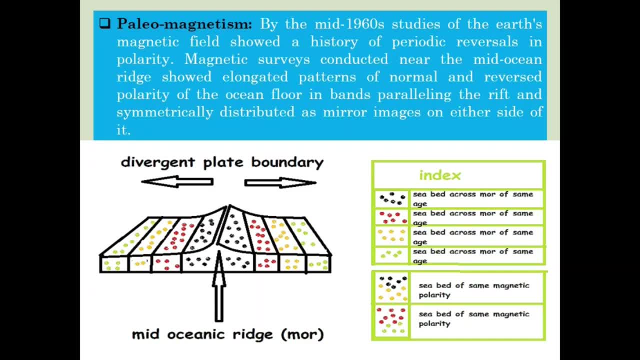 and which is more distant from the source, will have the negative in the north and positive in the sun. as the rule of magnetism, positive polarity will not allow new rock to form positive in front of them. they will force them to form negative polarity. on the other hand, negative polar 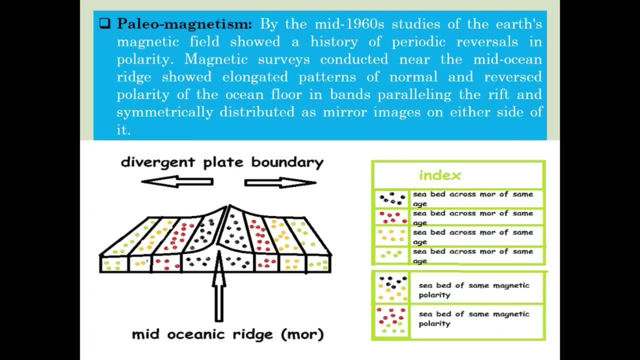 duty of the rock formation will not allow negative polarity to form close to them. they will force the new form, newly formed rock to be positive. like, like, exactly the same thing. we read in that different kind of charges will attract and similar kind of charges will distract each other. and because of that, with the difference in age and formation, 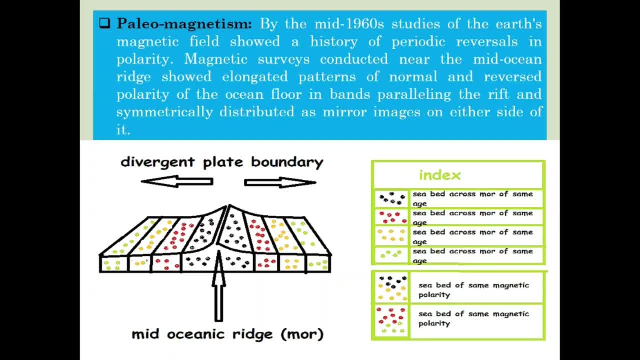 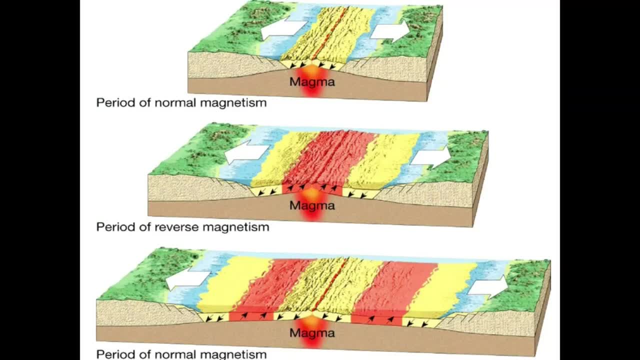 you will also find the inverse, or the reverse of the polarities in those rocks. so this is the same thing just elaborated in a more clear vision. you can see the colors. making and clear indication are that they also contain the same polarity, and all those arrows will give you the different polarities. 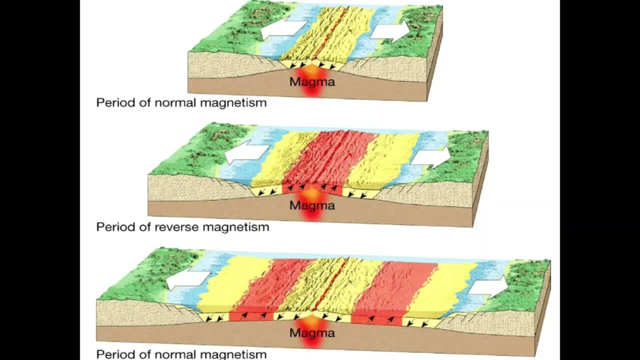 direction of the polarity. so if the yellow one is positive and negative at first, so the second one, the younger one that comes later, the red one, it will have negative and the positive exactly opposite to their, uh, to their corners, and after that, if there is another formation, then it will have again the 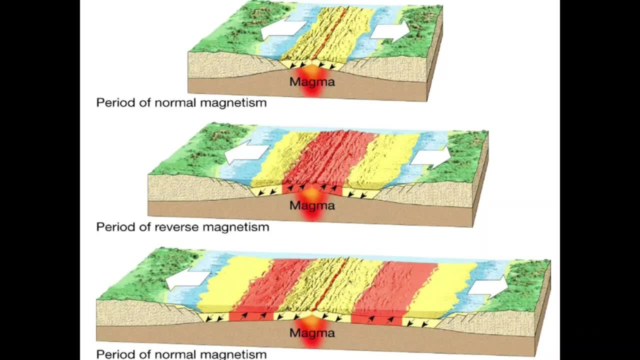 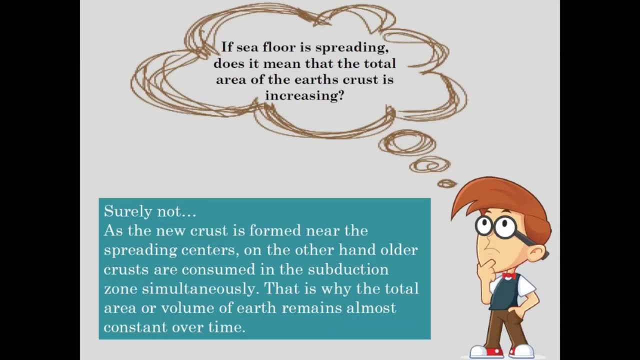 opposite of the previous one, and this is how the formation will continue and continue and continue to spread. so now there is a question: if sea flow is spreading, does it mean that the total area of tart's crust is increasing? surely know that we already mentioned that in one portion, from one part, due to the 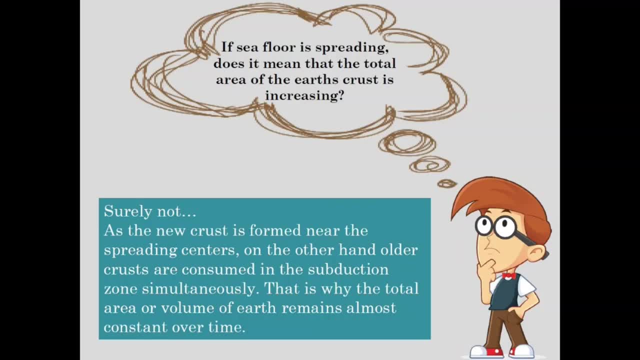 uh, opposite direction of convection. sea floor is spreading, new magma is coming to the top and forming new rock formation, forming new crust. but on the other hand we also see in the other side, or in both other sides, uh, for similar kind of convection: plates are going beneath each other, plates are going 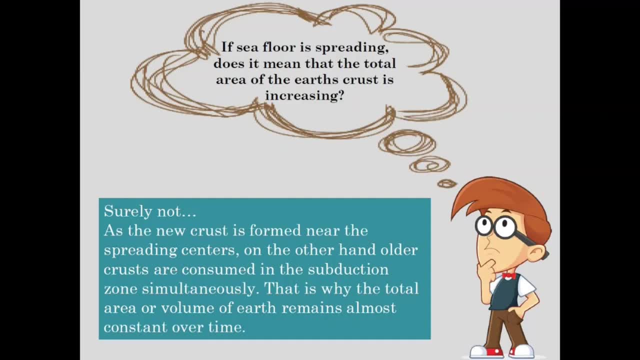 subducting into the mantle and same or almost similar amount of crust is being turned into liquid magma again and getting inside the earth's internal formation. so there is always a balance between this new formation and it is the melting of orderly formation, that crust. so that's why the total volume or total area surface. 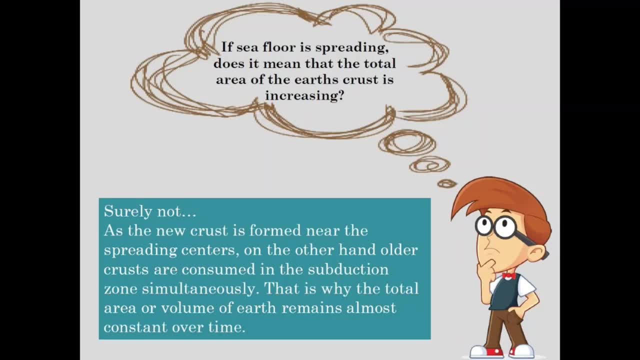 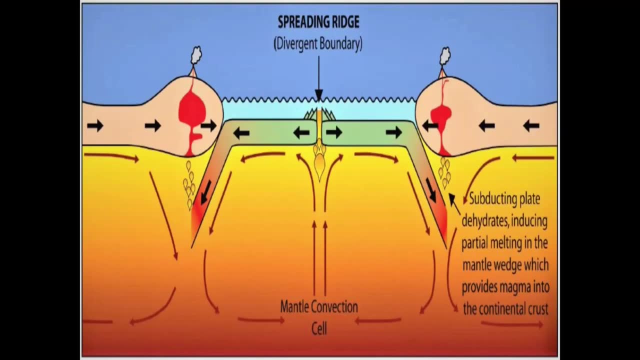 area doesn't usually increase or decrease, even if it is, but it's not that much noticeable. so this is another picture detailing everything in clear physics that you can see: the mental convection cells: they are pushing the place. on the other hand, the similar direction convections- they are pushing the oceanic crust. 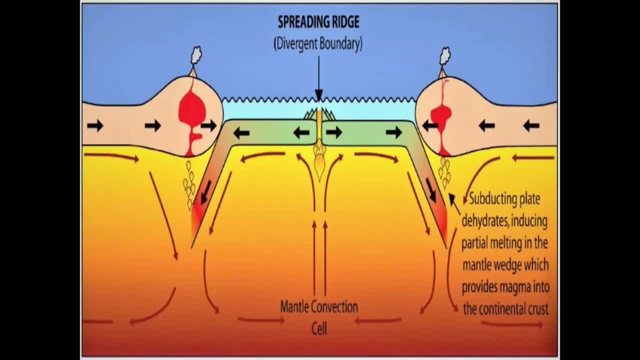 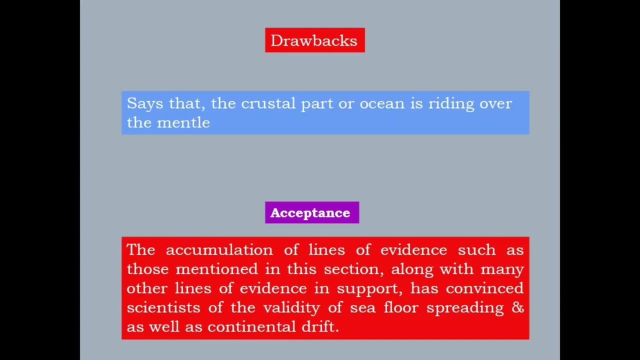 down beneath the terrestrial crust, and that's why, if one place there is a deformation, in the opposite there is a deformation or there is a distraction of the previous crust. now, this theory also had some drawbacks. what is that? the crustal part of ocean is riding over the mantle. 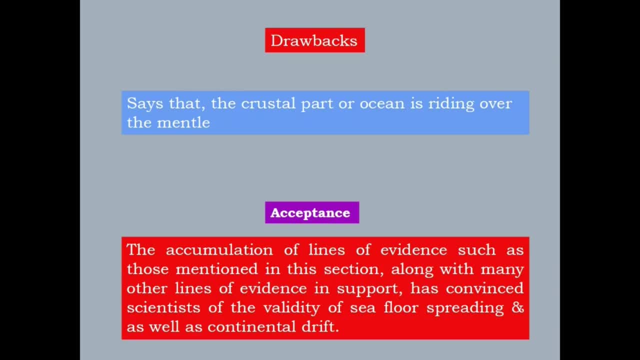 that okay, and uh, everyone is asking that okay, if the crustal part of the ocean is sliding over the mantle, how? how does that even possible? so the accumulation of lines of evidence such as those mentioned in the section, along with many other lines of evidence, is supposed has convinced some of the group of 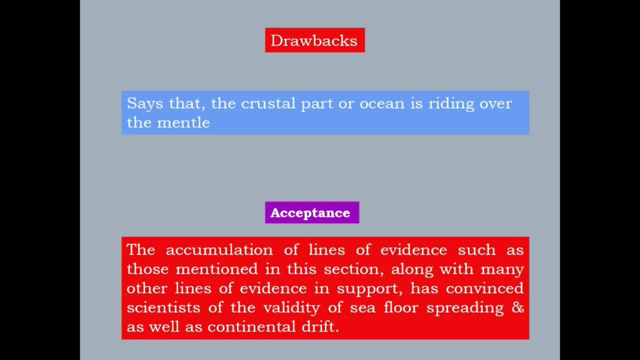 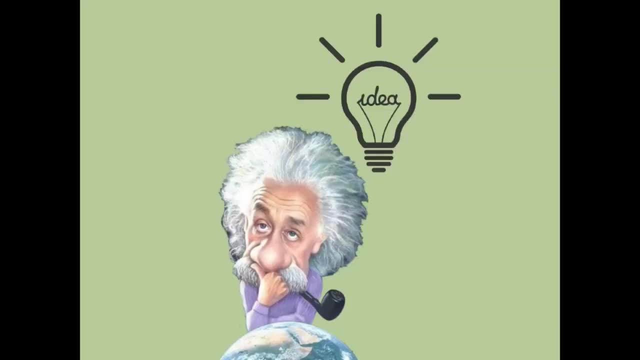 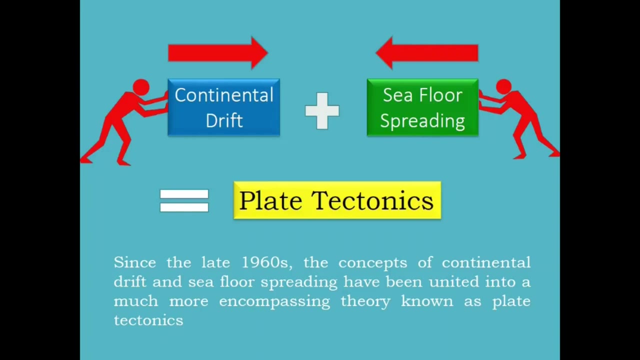 scientists of the validity of sea floor spreading as well as the continental drift. but still there were questions. and later, what scientists do they have an idea? they have an idea to combine both the theories and turn them into one. in that endeavor, they just tried to make a connection between both the theories and finally, 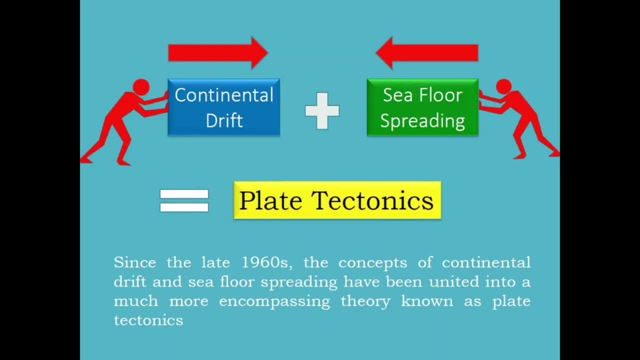 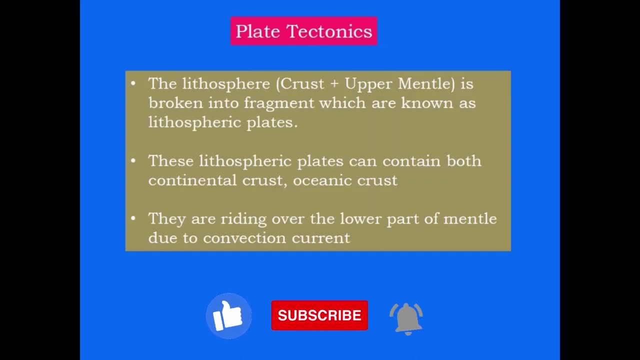 they come with the split tectonic theory in 1960s that the lithosphere, that means the crust and the upper mantle, is broken into fragments which are known as lithospheric plates. it's not always oceanic crust or terrestrial crust or continental crust. it's we call it lithospheric plates that. 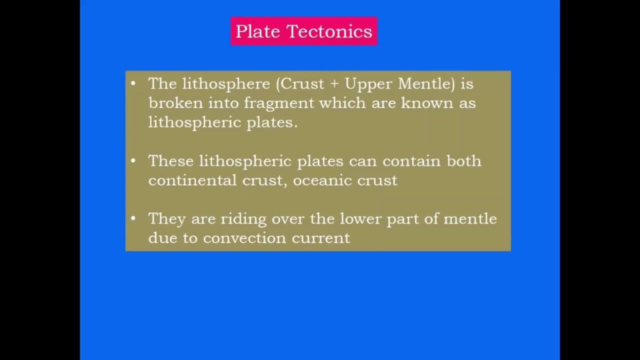 consist both the crust and the upper mantle. they are not separate units, but they're the same unit. as together, then these lithospheric plates can contain both continental crust as well as oceanic crust. they are riding over the lower part of the mantle due to the convection current. 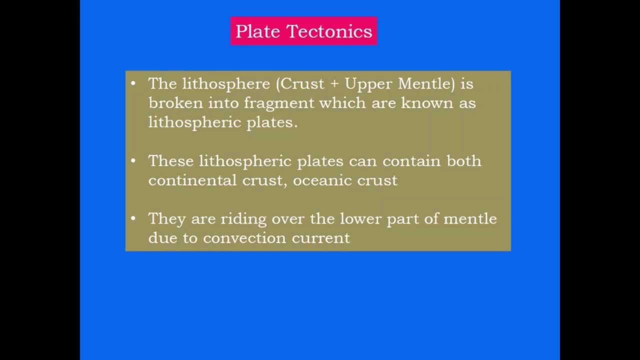 even though they're same information, even though they are considered as one unit. but still the mantle is liquid and the crust is not liquid, is solid, so that is why it is riding on top of the mantle. so if we consider this- both the thing, the mantle and the crust- as one unit, then we can find the validity. 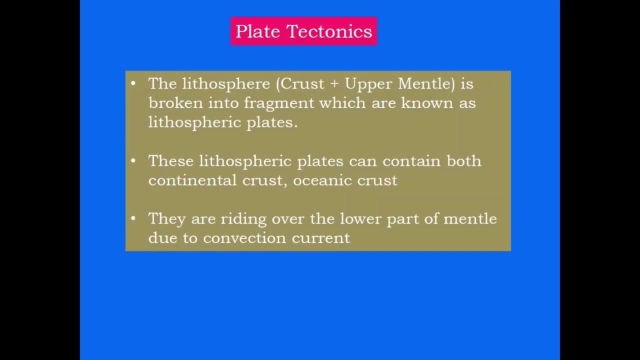 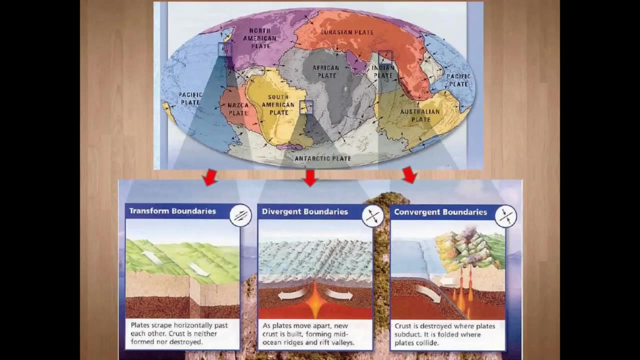 of the sea flow is spreading as well as the continental drift. now let's discuss the plate tectonics. in very brief, the plate tectonics mean that our plates, all these lithospheric plates, the composition of mantle and crust. they are not like steel, they're dynamic and their dynamics have different kind of 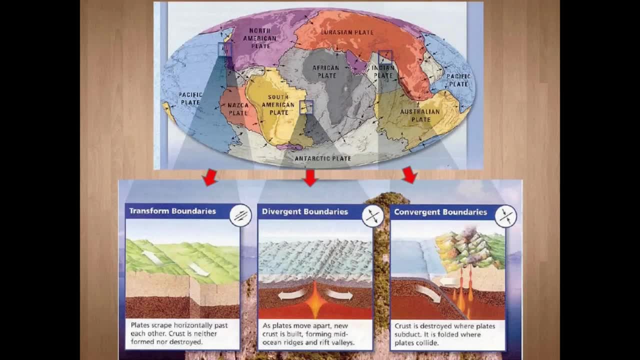 situations. for example, plates are not always moving towards each other, not always moving away from each other, but they are also moving side by side. so when the, when two plates moves away from each other and forms new plates, that movement is called divergent movement and because of that movement, the boundary that we get in the source, that 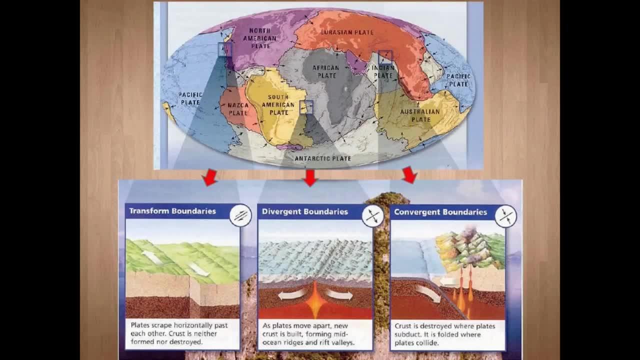 we call it divergent boundaries. on the other hand, plate that morphs towards each other and creates these elevations in the earth's crust and the oceanic and the destruction of oceanic crust. this kind of movement is known as convergent boundaries. on the lastly, there is another specific kind of movements. 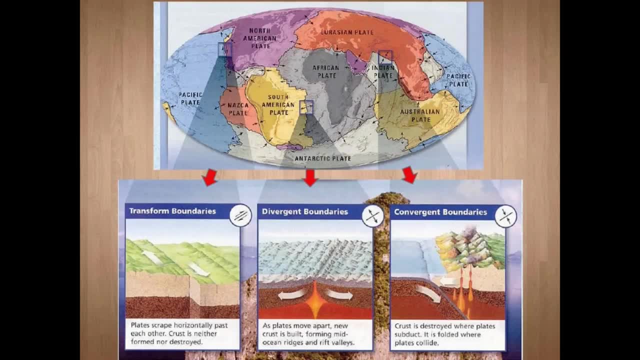 like movement side by side. for example, one plate is moving upward and one plate is moving southward- not exactly upward or southward, it would like one plate is: if one plate is moving north, then another is moving south, and if one plate is moving in the east, 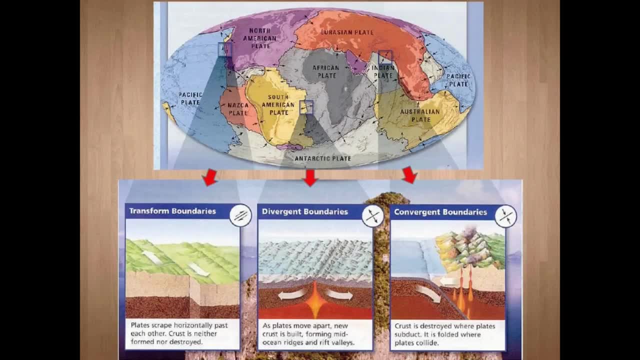 other is moving in the west, so completely opposite towards each other, and that creates another kind of boundary known as transform boundaries. okay, so these are the major three boundaries that were created in the first place and that was finally came up, finally discovered by the scientists, and that supported the idea of both the sea floor spreading. 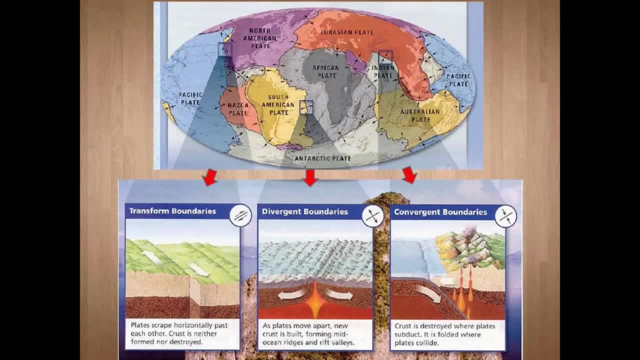 and continental drift. after this idea, all the previous little ideas which are rejected initially or not accepted directly by the scientific community were finally accepted, and now we have this new uniformed theory known as the plate tectonics. so this is all for today. maybe in another lecture